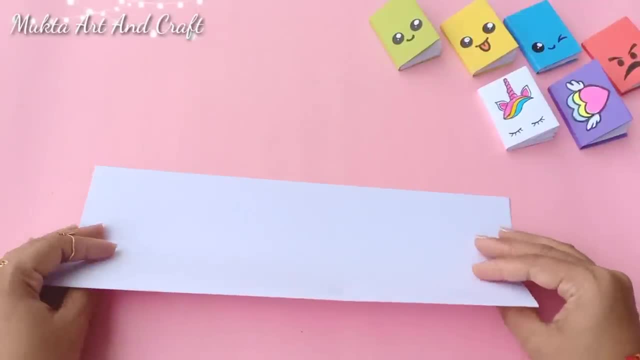 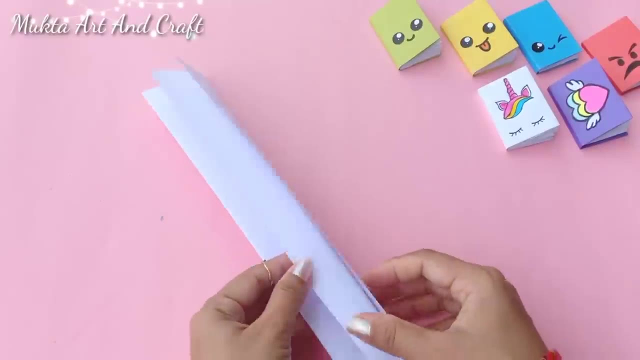 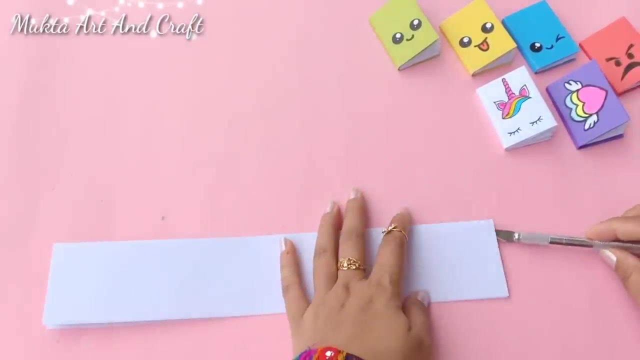 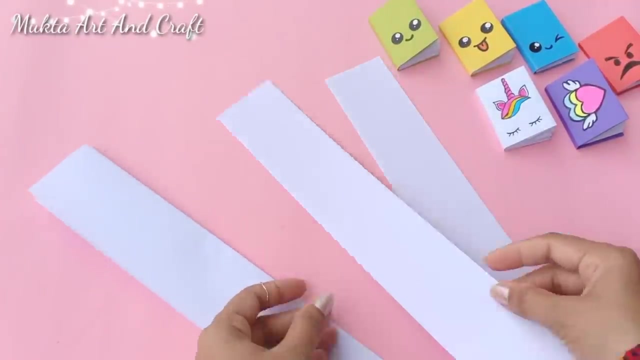 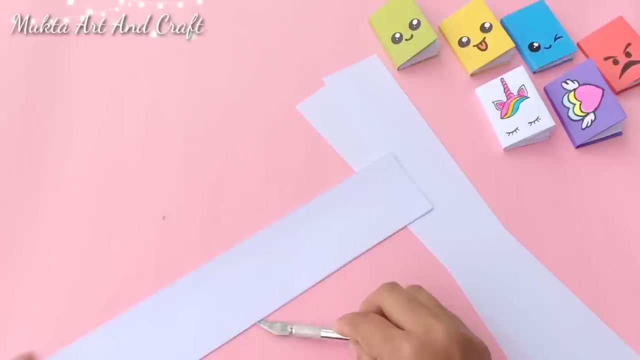 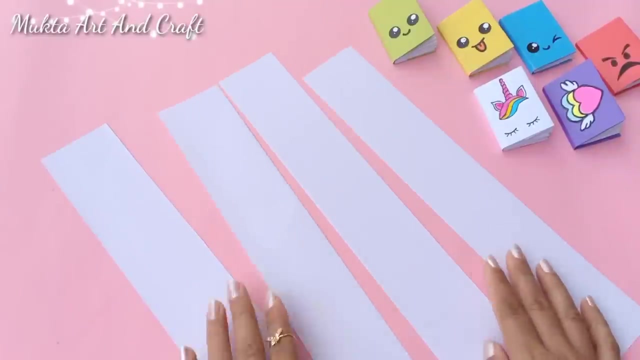 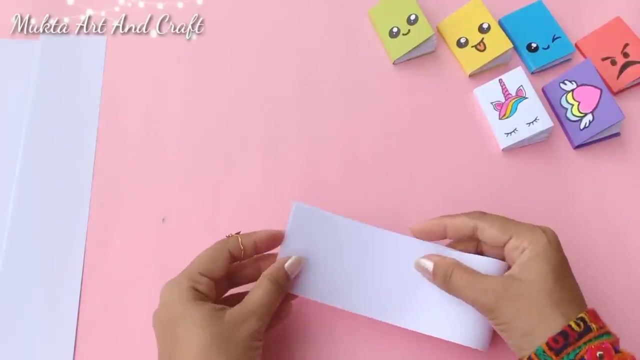 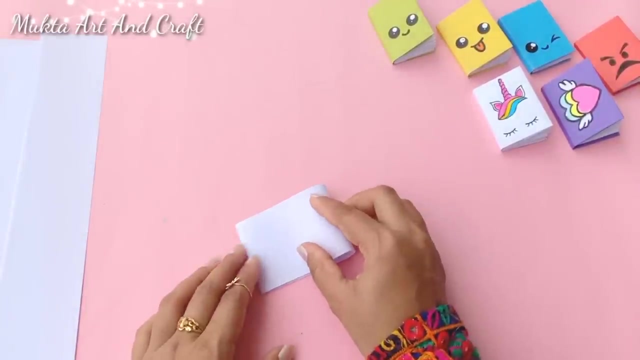 If we never see tomorrow, babe, if we never make it through today, If we never see tomorrow, babe. I know that I lived how I wanted to, Don't want to, Don't want to, Don't want to. The lights in here are blinding me and I can't see clearly. 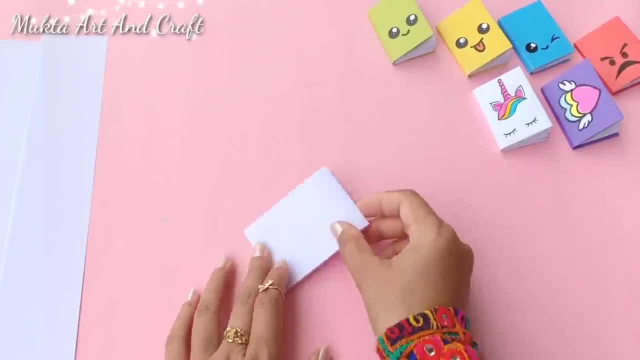 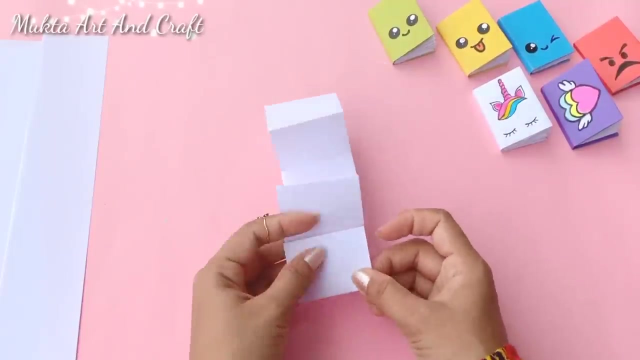 I have no fear how this will end. no, nothing scares me anymore. The lights in here are blinding me and I can't see clearly anymore. I have no fear how this will end. no, nothing scares me anymore. If we never see tomorrow, babe, if we never make it through today. 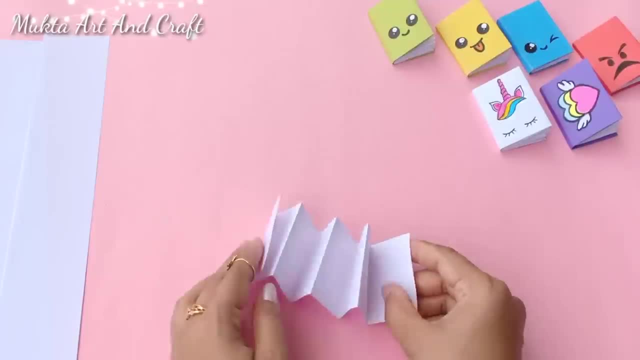 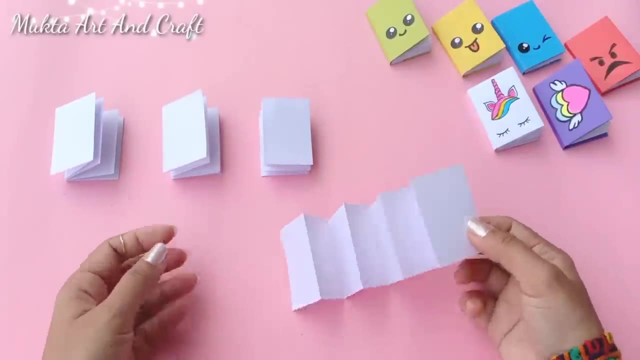 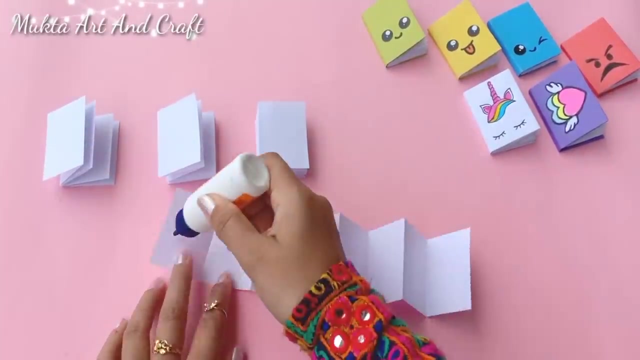 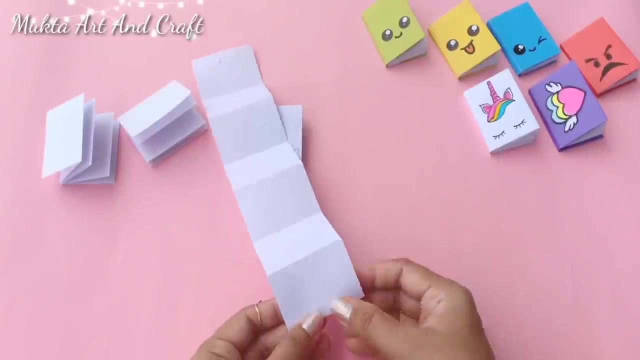 If we never see tomorrow, babe, I know that I lived how I wanted to. If we never see tomorrow, babe, if we never make it through today, If we never see tomorrow, babe, I know that I lived how I wanted to, Don't want to. 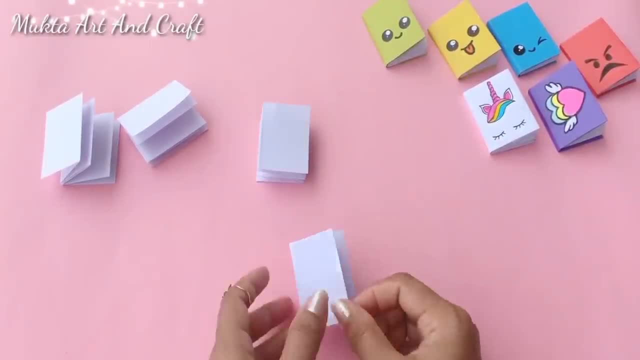 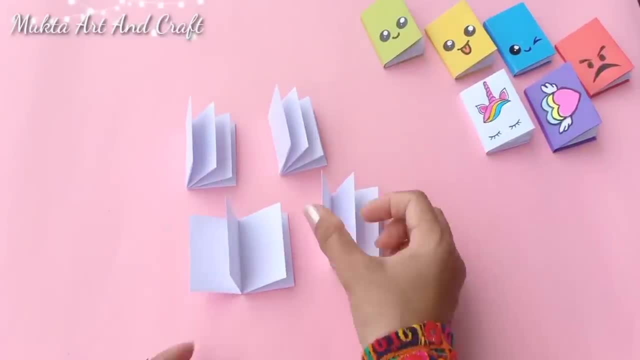 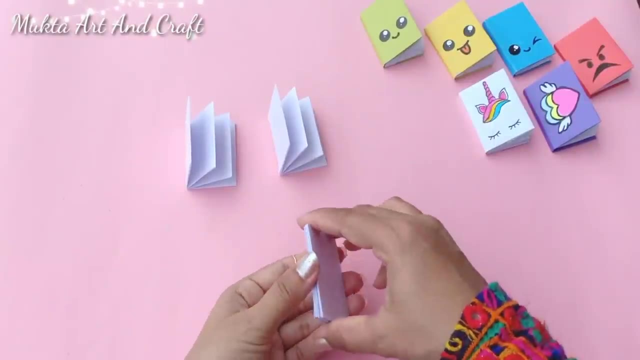 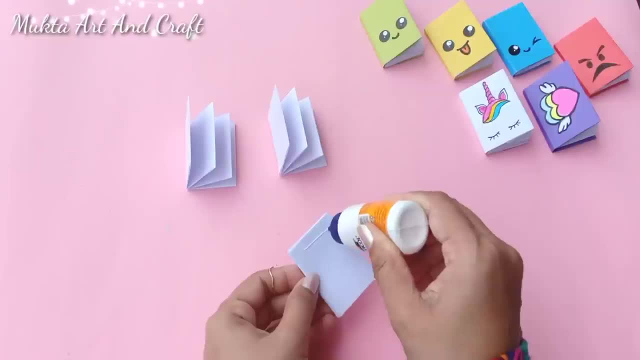 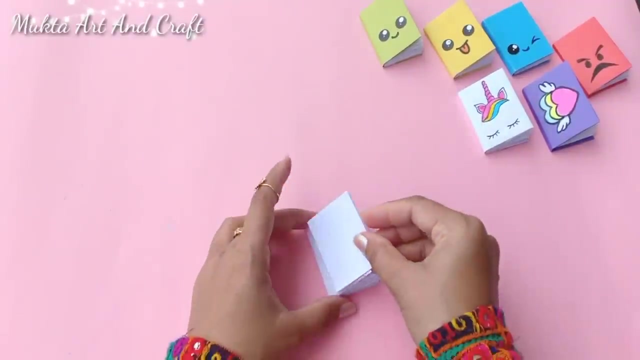 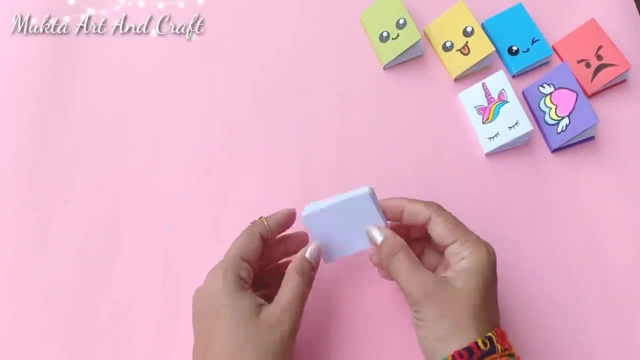 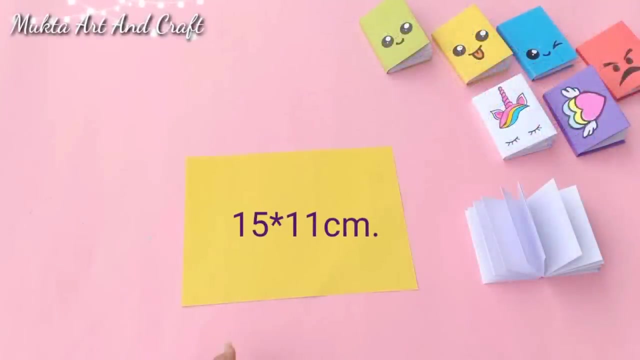 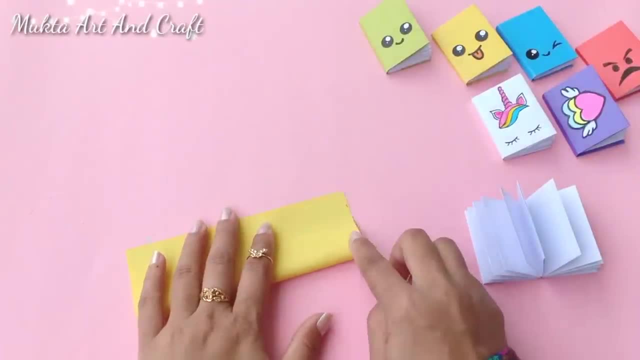 Oh, and if you love me, baby, say it now. Oh, and if you love me, baby, show me now. Baby scream it loud. So just say it now, Baby scream out loud. So just say it now, Baby scream out loud. 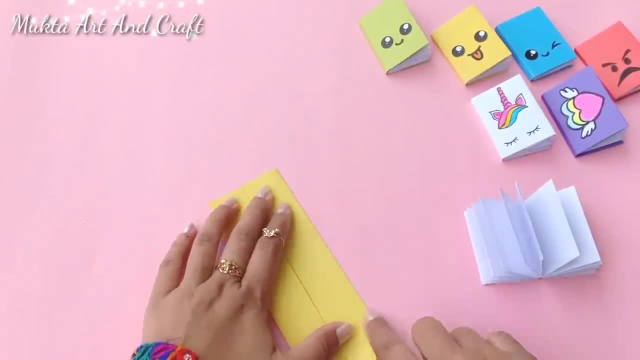 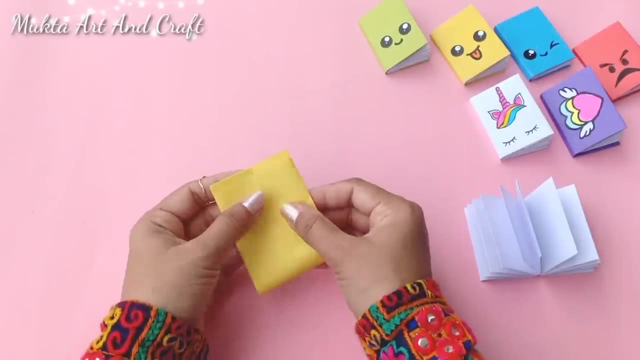 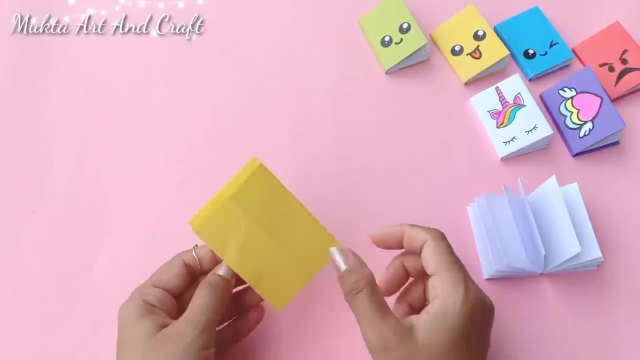 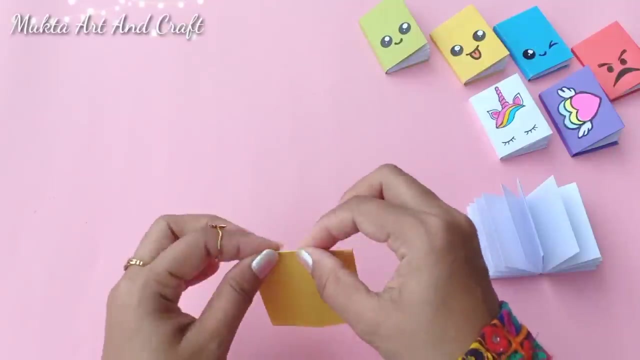 Baby, say it now. Baby scream out loud. So just say it now. Baby scream out loud. If you want me, baby, let me know now, Oh. and if you want me baby, show me now, Oh. and if you love me, baby, say it now. 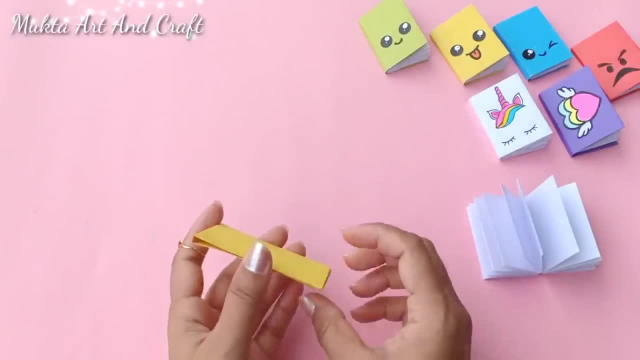 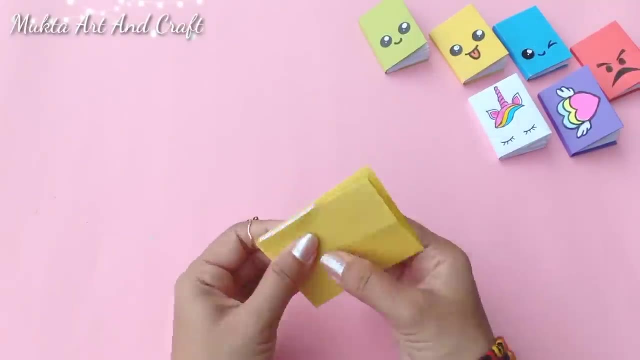 Oh, and if you love me, baby scream it loud. So just say it now. baby scream out loud. So just say it now. baby scream out loud. Baby say it now. baby scream out loud. So just say it now. baby scream out loud. 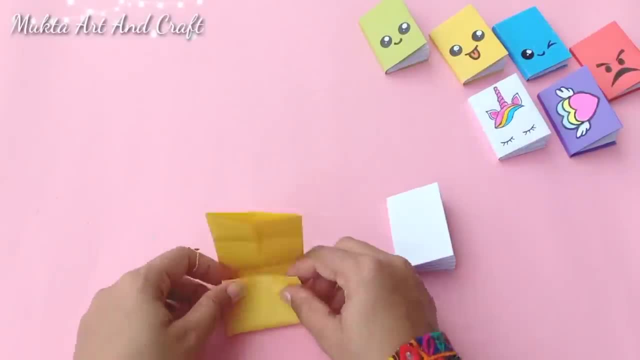 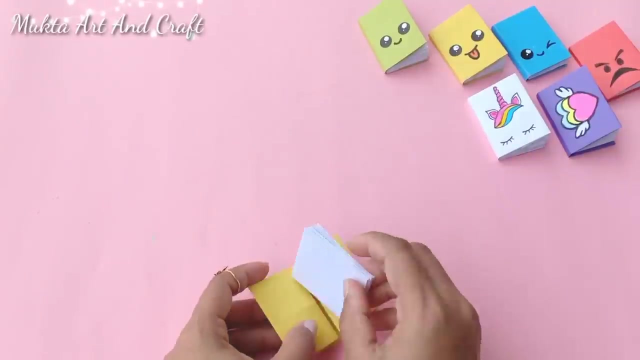 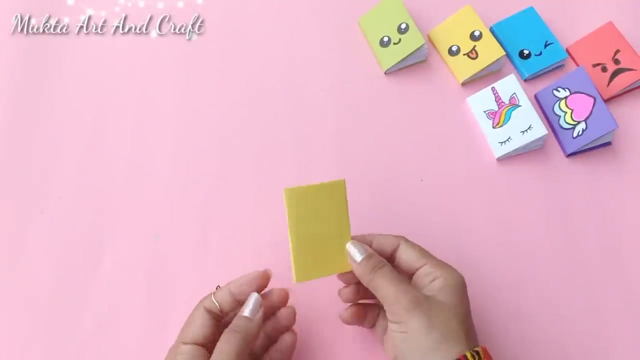 Baby, say it now, baby scream out loud. So just say it now, baby scream out loud. Baby say it now, baby scream out loud. So just say it now, baby scream out loud. Time after time, you're always right, You never chase. yet hold me tight.